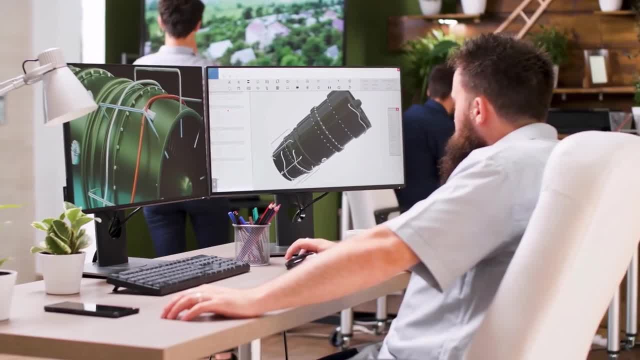 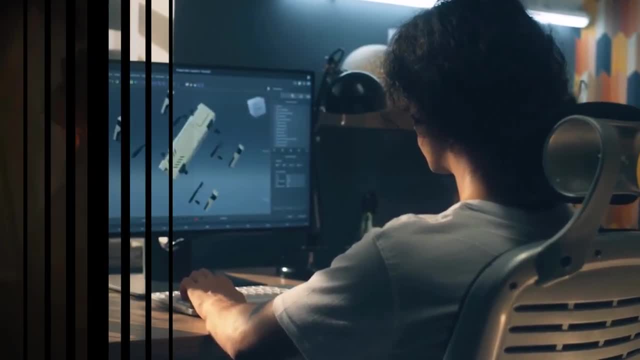 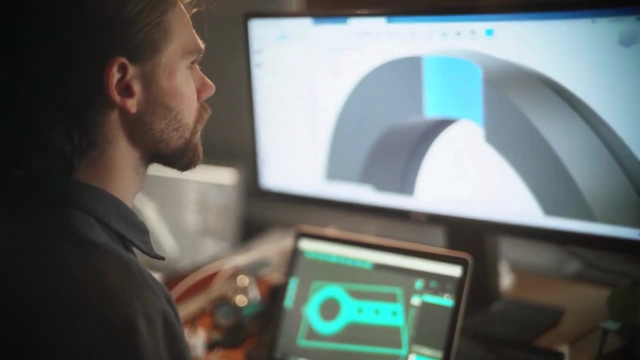 exploded views for presentations, reports, price calculations etc. and being articulated, and the assembly terminology was really helpful. There are many available CAD software on the market, but for purpose of this video I will use Autodesk Fusion 360.. However, I will try to keep. 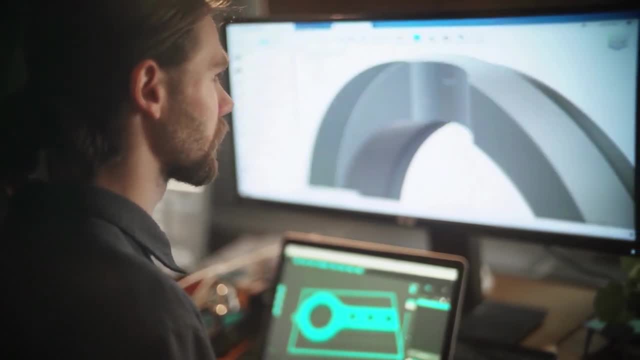 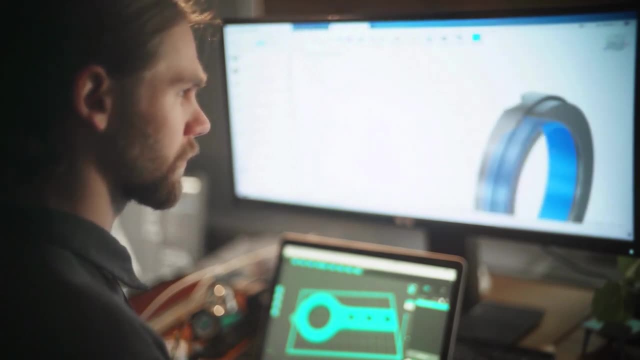 the video as generic as possible so that you could apply the knowledge to any other CAD software. In my opinion and experience, once you learn how objects are made in 3D environment, you understand the general logic of CAD software and you learn to work in one CAD software. 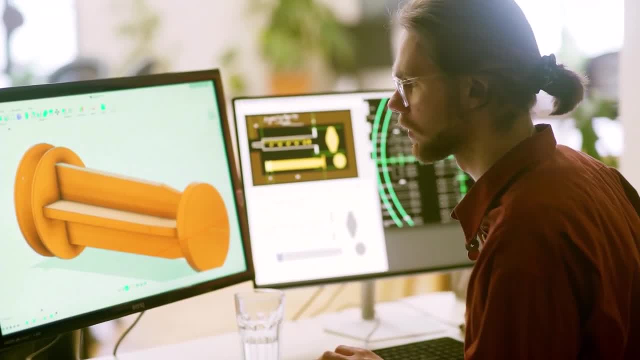 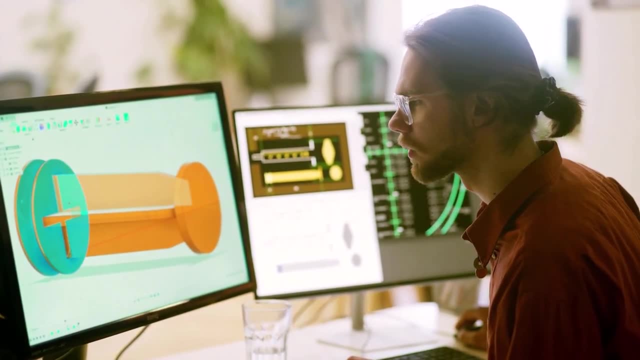 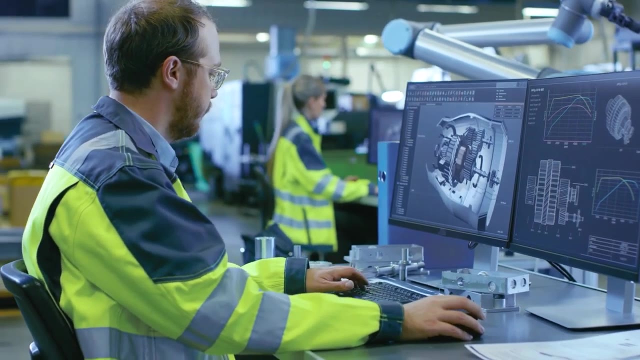 you can learn with ease any other CAD software on the market. I will repeat myself again and emphasize that CAD software is tool that mechanical design engineer use to, based on mechanical engineering fundamentals, build real life solutions. CAD is extension arm of our knowledge of mechanical engineering principles. 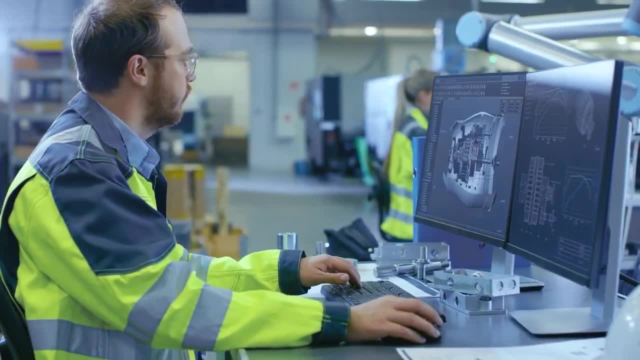 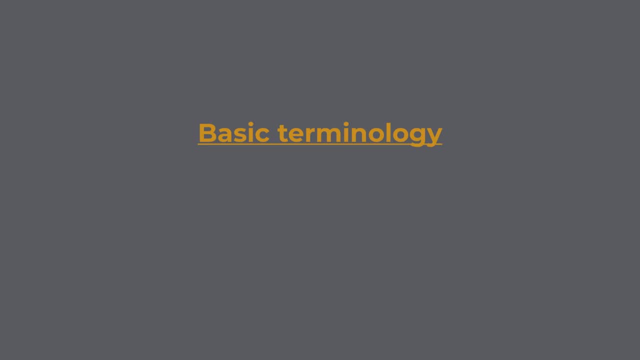 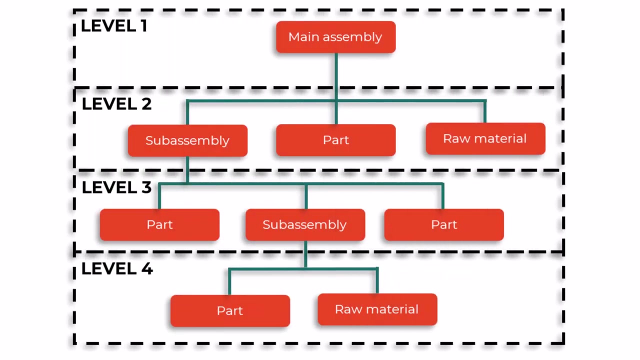 not the other way around. Keep in mind that software is only smart as the person using it. Basic terminology: Let us know. look into some of the basic terms that you will encounter when creating assembly in CAD software: Assembly subassembly, As previously mention, assembly is model that is build from two or more parts. 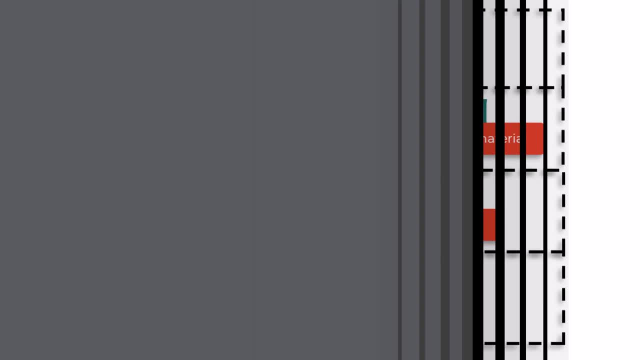 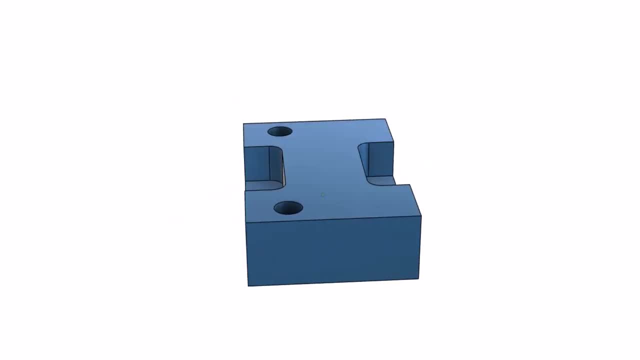 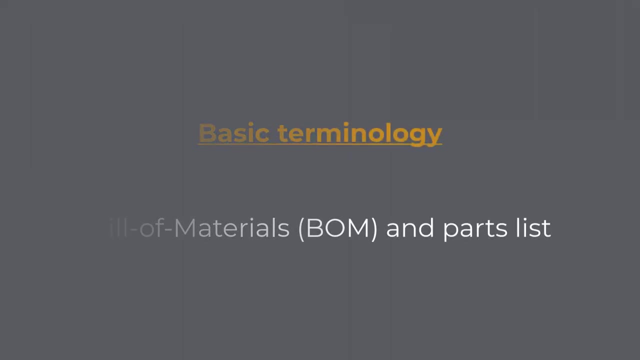 Subassembly is a smaller assembly that is part of larger assembly. Part According to ISO 298452011, part model is model in which the product described is one single item. We already cover this topic in depth. Bill of Materials, BOM and parts list. 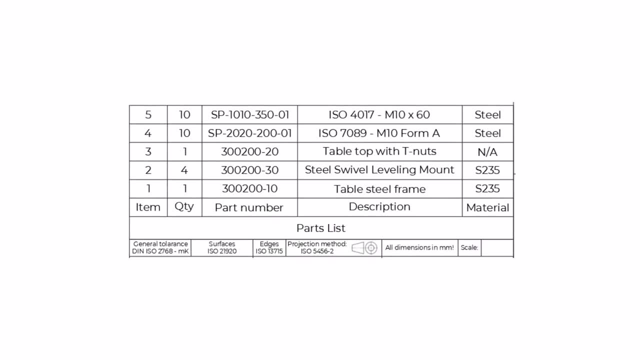 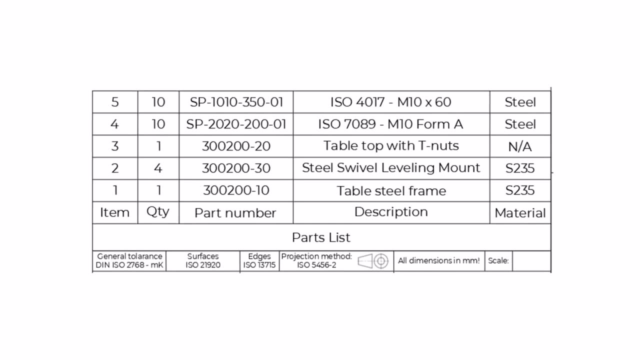 The bill of materials list the subassemblies, parts and materials required for building the assembly. The parts list, or BOM, can be added directly to the drawing or provided with the assembly drawing as a separate list. The difference between the parts list and BOM is that the parts list defines 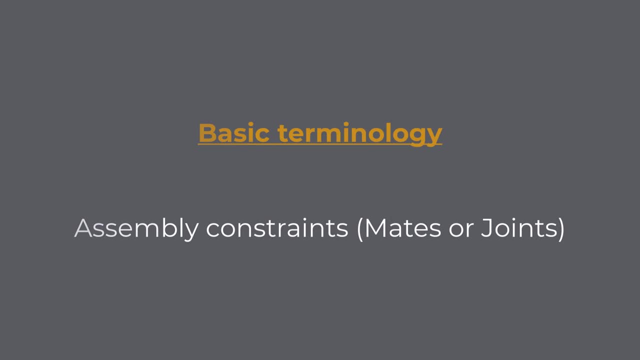 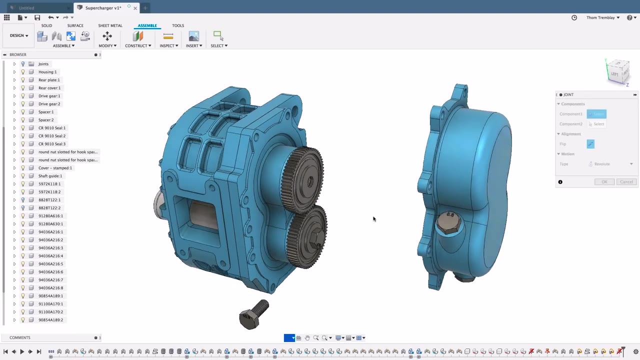 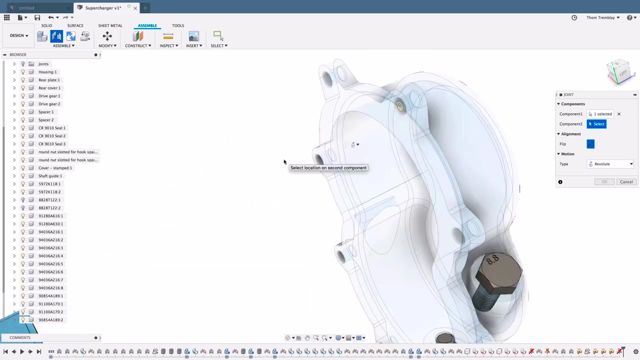 only one structural level. Assembly constraints, mates or joints. Assembly constraint is a type of constraint that defines the relationship between two components, specifying how they are connected or positioned relative to each other. Depending on the software, they can also be called mates, joints, constraints, etc. When we are defining the assembly constraints, basically we are: 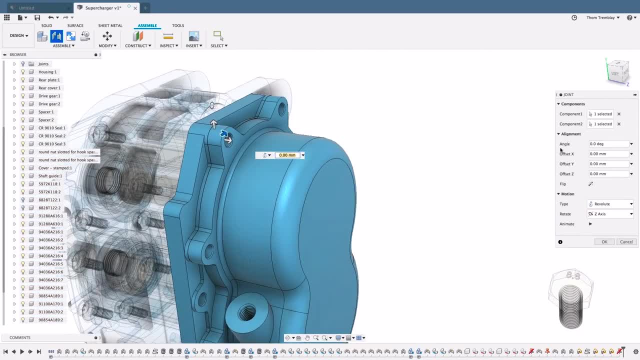 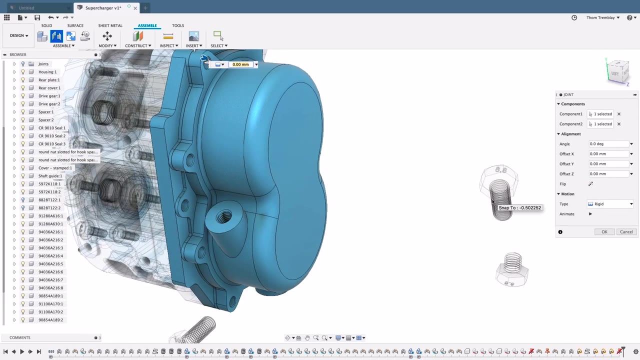 manipulating the degrees of the freedom of the parts. In the 3D space we have 6 degrees of freedom: 3 linear and 3 rotational. When the part has all 6 degrees of freedom, constrained part is considered fixed. Usually in CAD software the first component that is placed in the assembly. 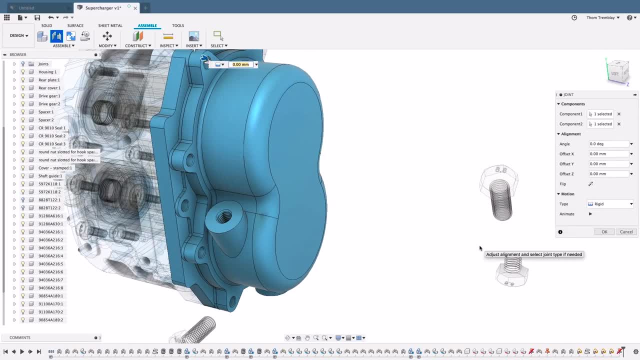 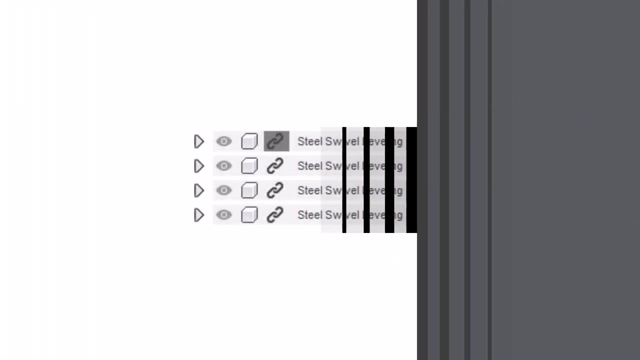 is fixed and then we are adjusting the degrees of freedom of other components in relation to the fixed one. Of course there is a possibility to define any component as fixed one. In Autodesk Fusion 360, assembly constraints are referred as joints Component instance When we have a component used multiple. 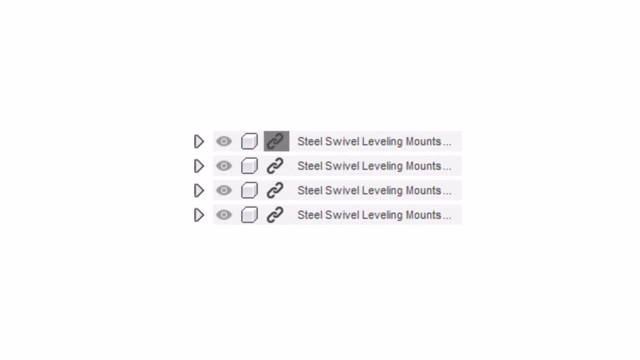 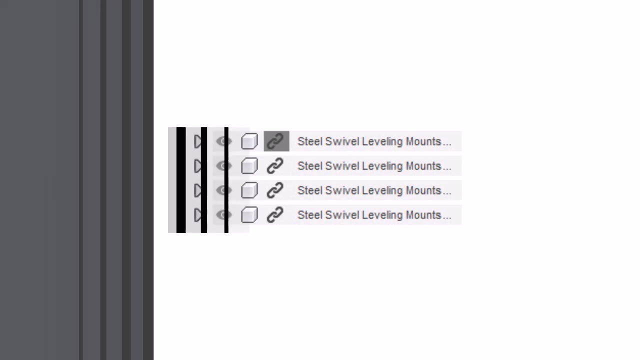 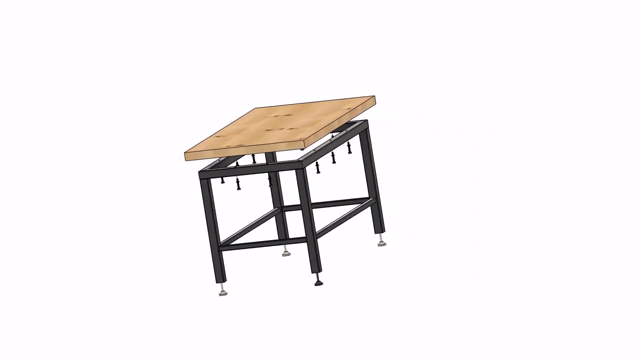 times in the assembly. this multiplied component is called an instance. The instance shows the same form on a new location in assembly as the original component, but it is not duplicated in the database. Exploded view. The exploded view illustrates the relationships between different components that form an assembly. 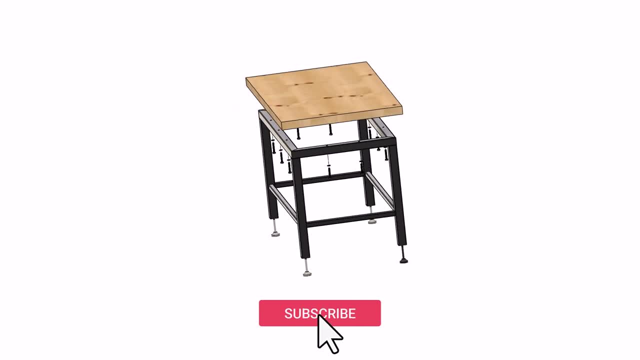 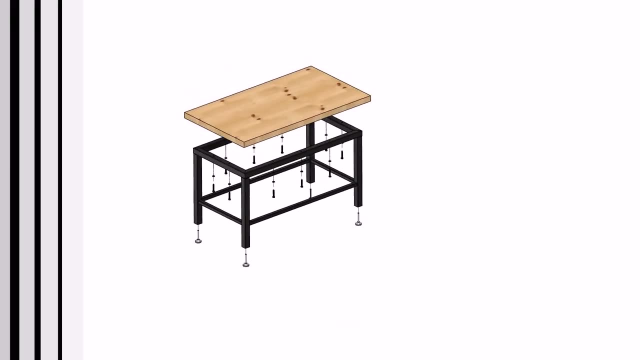 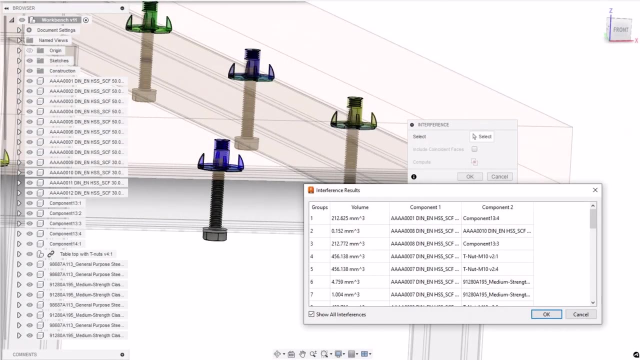 In other words, the exploded view shows how various components are put together to form the assembly. If you are interested about learning more about exploded views, check projection methods on engineering drawing. Interference and clearance. Interference occurs when two or more components within an assembly occupy the same space or overlap with each other. 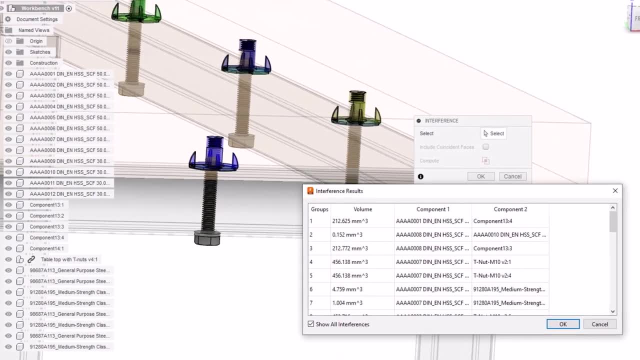 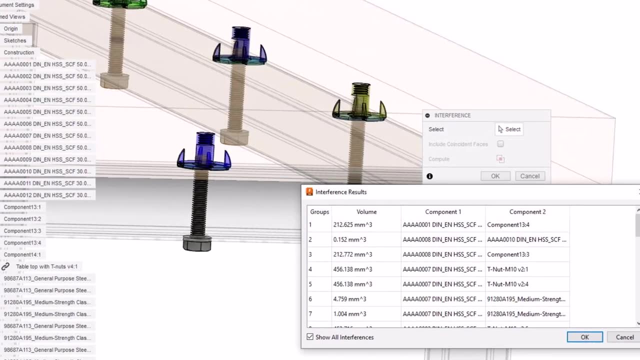 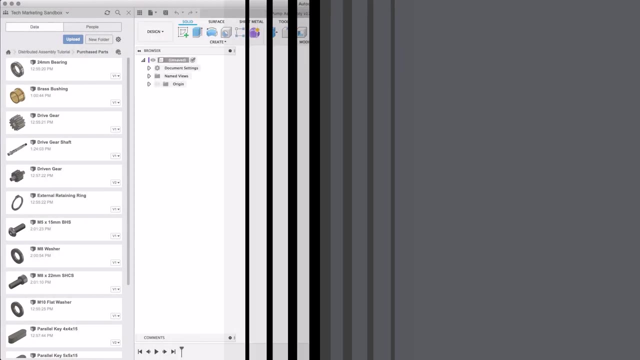 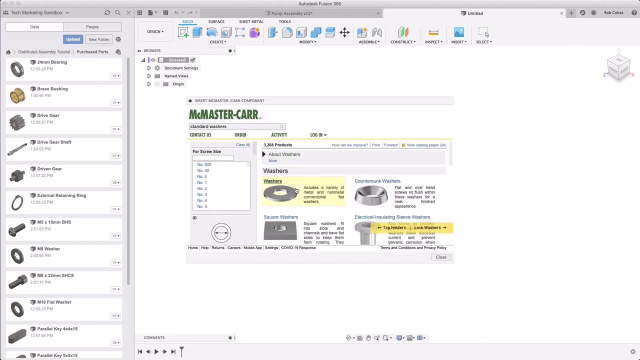 Clearance, on the other hand, is opposite. It is important to identify and resolve interferences to ensure proper fit and functionality of the assembly. Part libraries- Part libraries are collection of pre-designed and standardized components within CAD software. We also call them part catalogs. When we are working with assemblies, a lots of 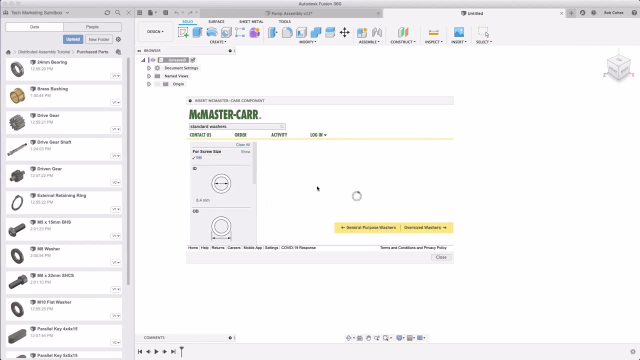 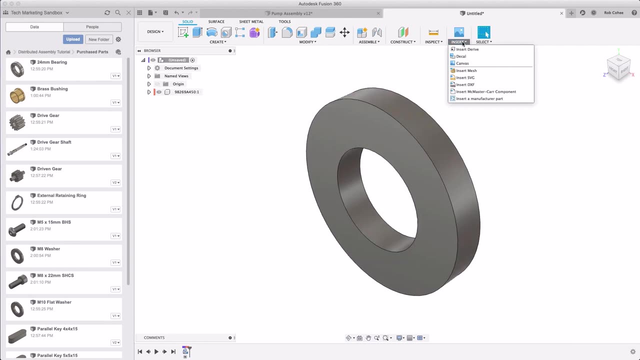 times we will use standardized or vendor parts, like, for example, screws. Instead, we create the screw part each time we need them. we will create them one and then save them into our part library. Part libraries. Part libraries are a collection of pre-designed and standardized components within 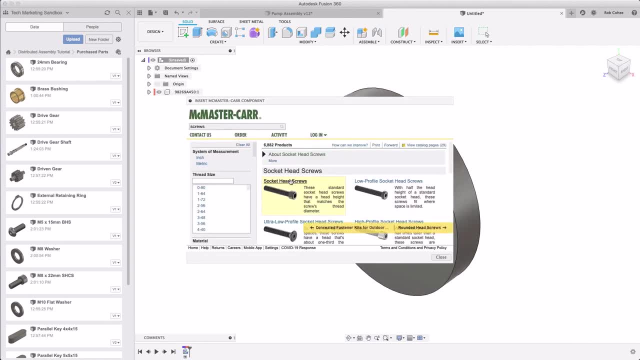 CAD software. We also call them part catalogs. When we are working with assemblies, a lots of times we will need this part. we can just reach into our library and use it directly in our assembly. Same things goes for often used supplier parts. Ideally, we will not create standardized part. 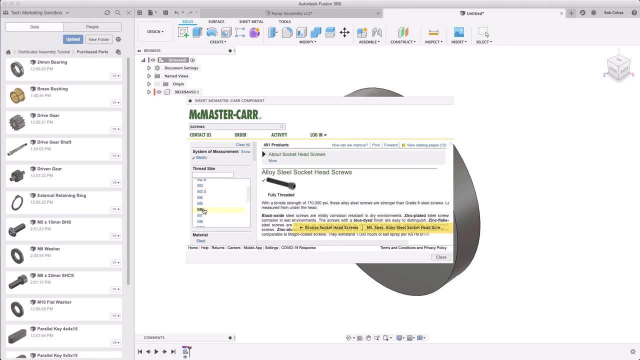 each time we need. instead, we will import the part library that was previously created by some other company or individual. There's a lots of websites on internet, but the most popular are grabcad, traceparts, threedcontentcentral, mcmastercar and cadean's paart solutions Furthermore. 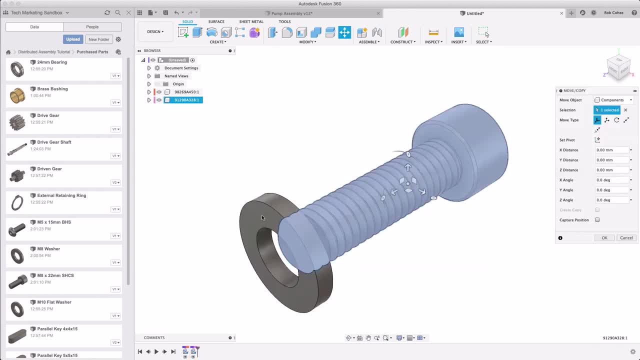 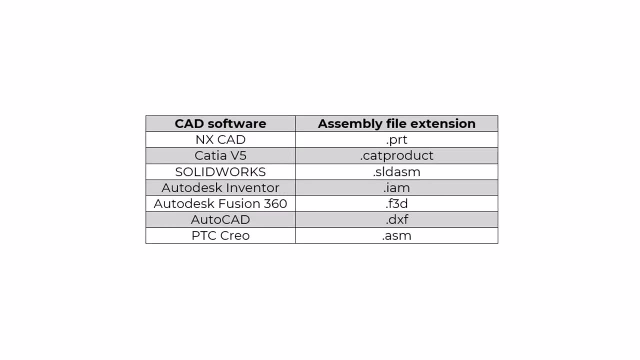 depending on the supplier. some of the parts are not standardized. If we want to import a part library from a supplier, sometimes you can find directly on their website 3D data for part you need, or you just ask them Part file types. Usually each CAD software has its own file formats that. 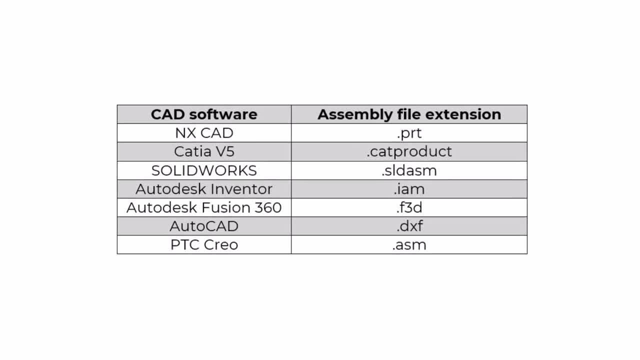 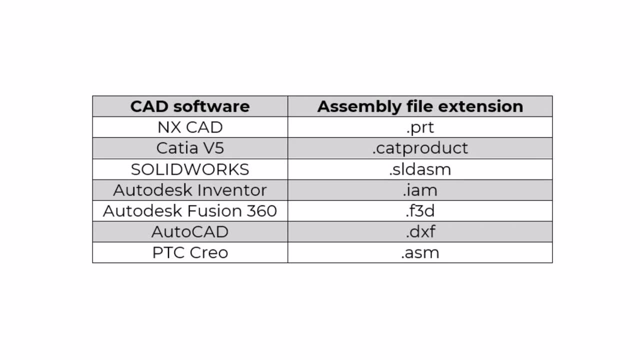 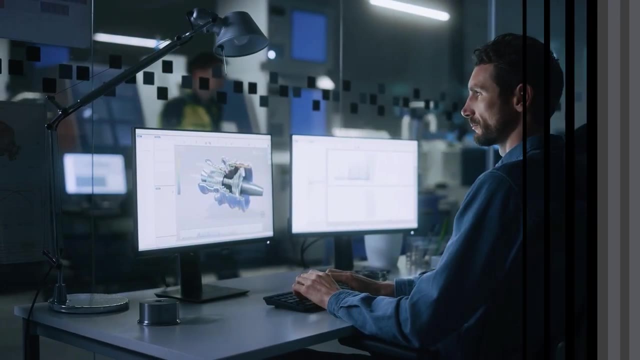 they are using to store relevant design and manufacturing data. Let us now look into some of the most known CAD software on market and their file extensions used to store assembly data. Assembly modeling techniques For assembly modeling. which type of part modeling is needed? the type of part modeling method we use is not important. Normally usable parts ends up. 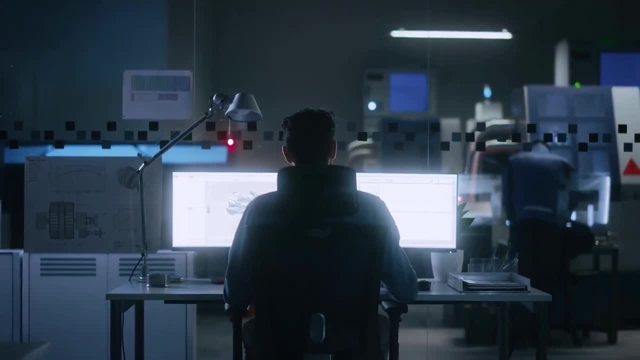 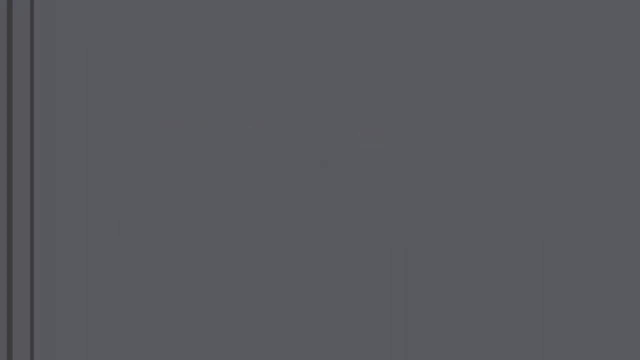 converted in solids anyway. Once. when we need to make assembly, we can use two modeling methods to do so: bottom-up and top-down assembly modeling. Bottom-up assembly modeling: In bottom-up modeling, first we create all the individual parts and then we build sub-assemblies, if any, and then finally. 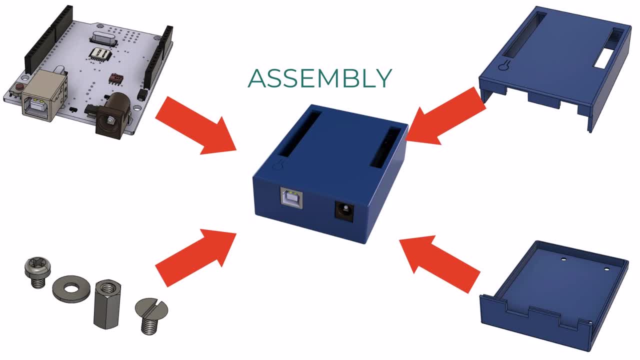 our main assembly. The final geometry of the product is not defined until we bring all the parts in the assembly. The final geometry of the product is not defined until we bring all the parts in the assembly. Assembly modeling- In top-down modeling we create overall assembly as one instance. 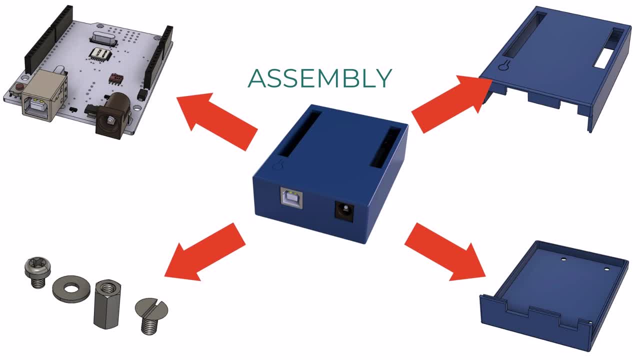 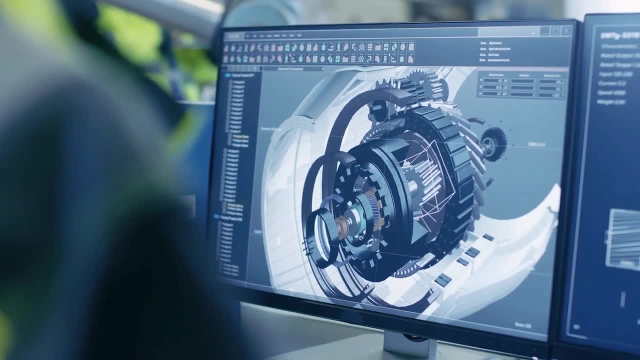 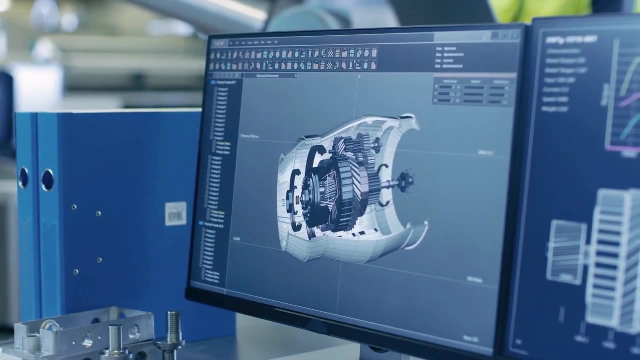 After the assembly is completed, then we create individual parts and sub-assemblies. that goes into the overall system. Usually we use combination of both methods. As a mechanical design engineer, knowledge of CAD is definitely required to land a job. Understanding and perfecting your CAD knowledge will definitely help you in a long run in your career. 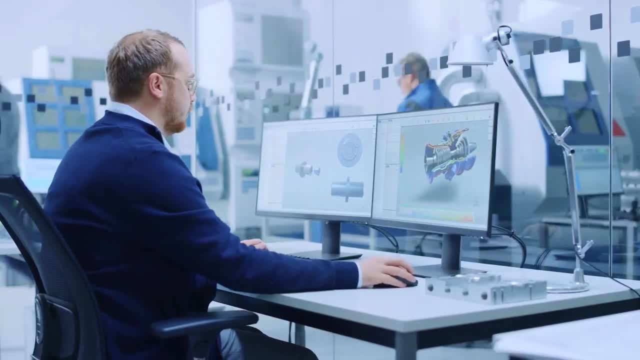 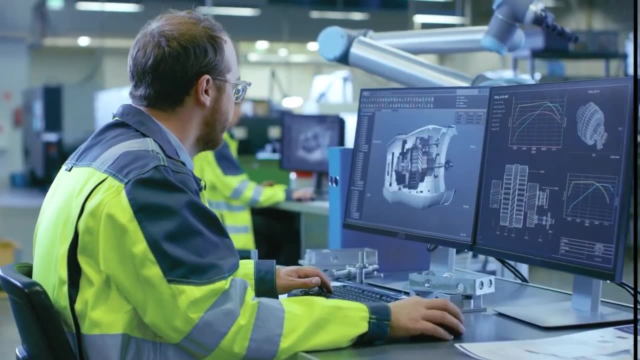 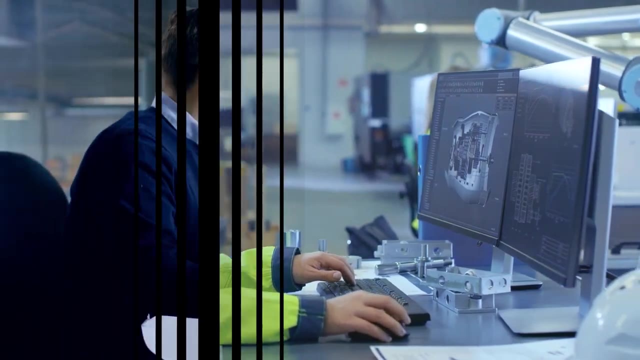 You will create assemblies often and from those parts you will create CAD drawings. Your drawings will be based on your assemblies created in CAD, so understanding the basics will help you in the overall design process. Using assemblies will be part of your normal job and it is good idea to spend some time understanding how it is properly done. 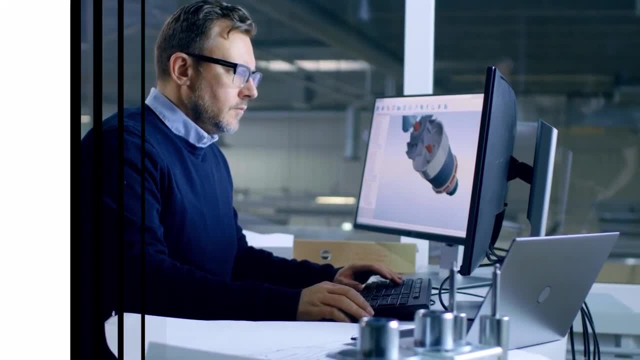 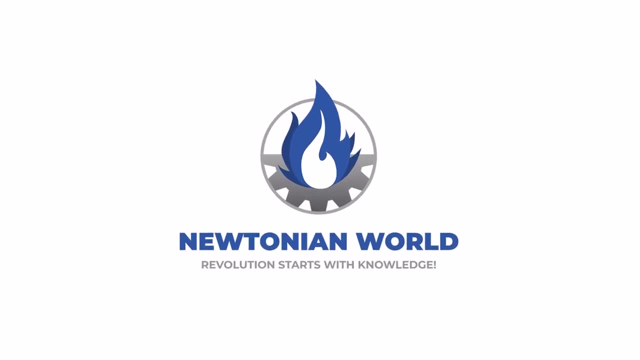 Because the CAD will be the tool that you will use very often, I would suggest you to spend some. Did you learn anything new in this video? Let us know in the comments below. Do you like our videos? Then give us a thumb up comment and share it with your friends. 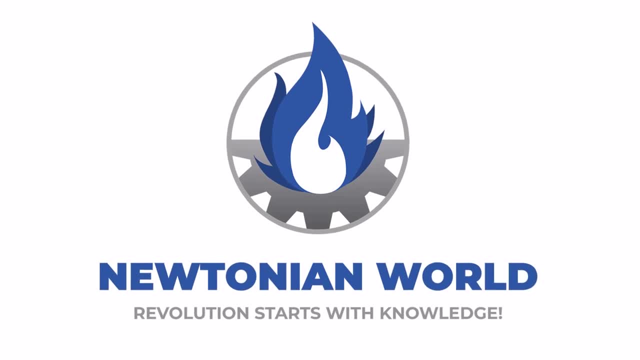 And if you want to become a part of the Newtonians, make sure to subscribe to our channel.